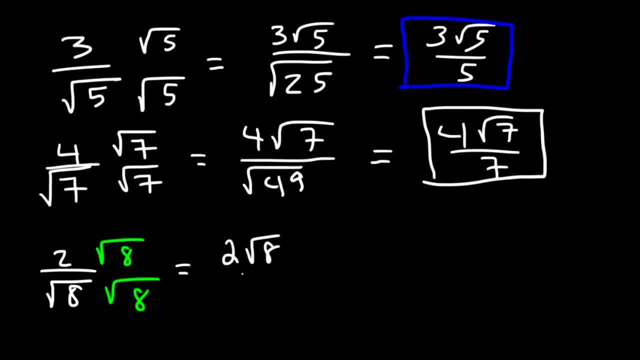 square root of 8.. So 8 times 8 is 64, and the square root of 64 is 8.. Now notice that we can reduce the fraction. We have a 2 and an 8. Both numbers are divisible by 2. So 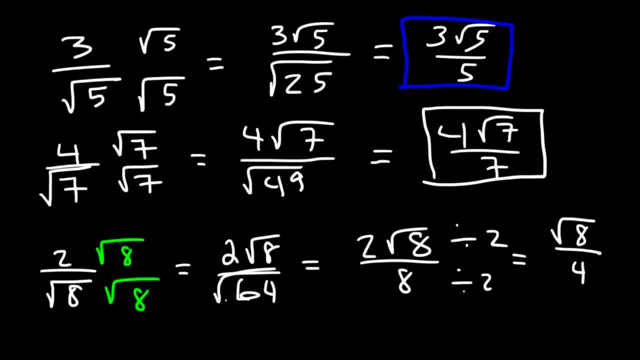 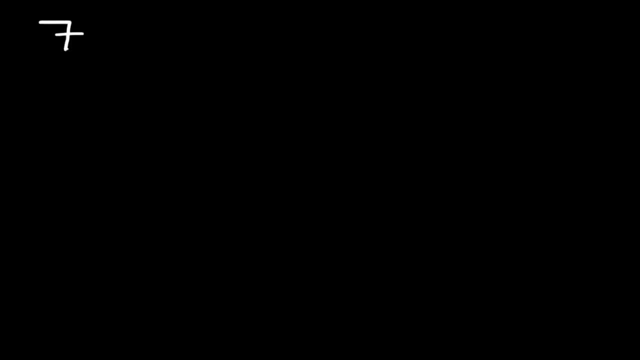 the final answer is the square root of 8 divided by 4.. Now go ahead and try these two examples. In the first example, we have an x instead of a number, But we're going to do the same thing. We're going to multiply the top and the bottom by the square root of x, So on. 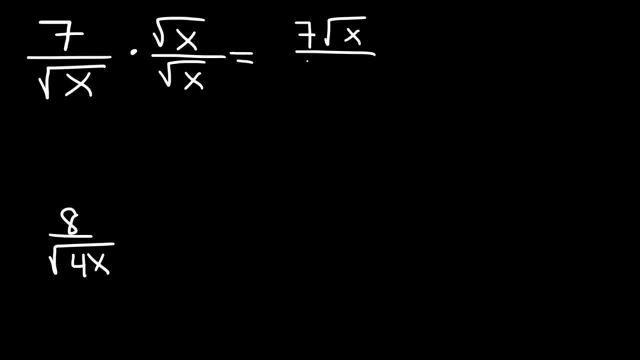 top it's simply 7 root x. on the bottom, x times x and the square root of x is 8.. So x is x squared And the square root of x squared is x. Now some teachers may require you to put an absolute value sign here, But I'm not going to worry about that in this video Now. 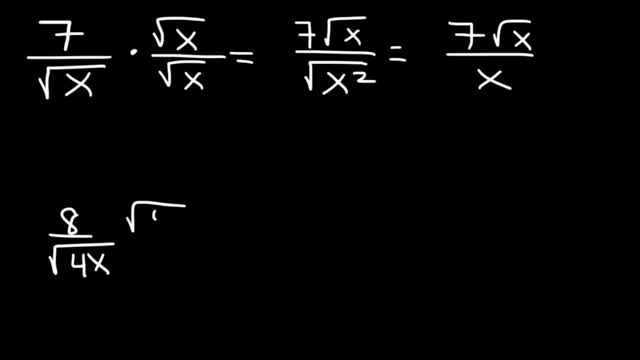 what about the next one? Let's follow the same steps. Let's multiply the top and the bottom by the radical in the denominator, So it's going to be 8 root 4x. 4x times 4x is 16x squared, And the square root of 16x squared is just going to be 4x. Now when you: 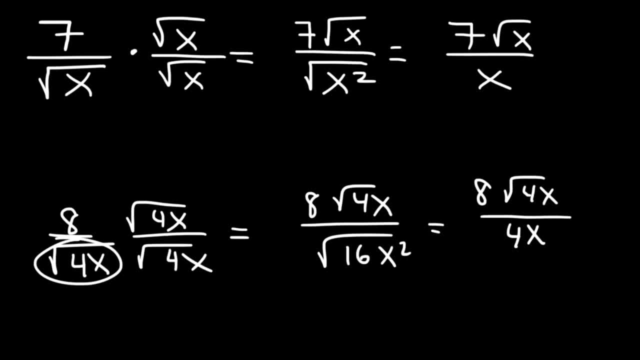 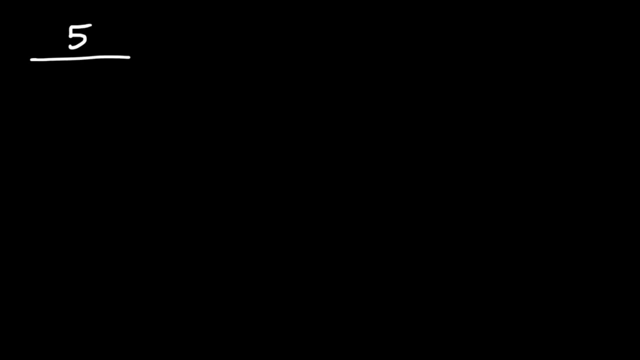 get to this point, always double check to see if you can simplify it further. We can: 8 divided by 4 is 2.. So the final answer is 2 square root 4x, 4x divided by x. Try this one: 5 divided by the square root of x to the 4th times y. 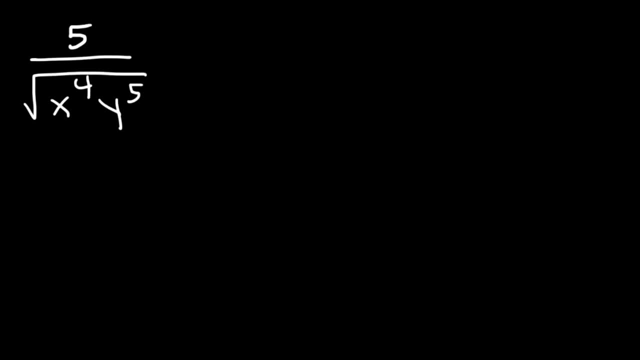 to the 5th. Go ahead and simplify the radical Now, before we try to rationalize it, we need to simplify the expression on the bottom. The square root of x to the 4th is basically x squared. 2 goes into 4 two times. Now 2 goes into 5 two times as well, with 1 remaining. So there's 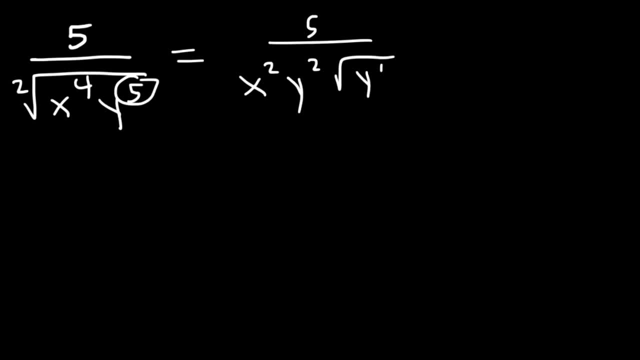 going to be a y on the inside. So now you want to rationalize the denominator at this point, after you've simplified first. So let's multiply the top and the bottom by the square root of y. Our goal is simply to get rid of the radical on the bottom, So we're going to have 5 root. 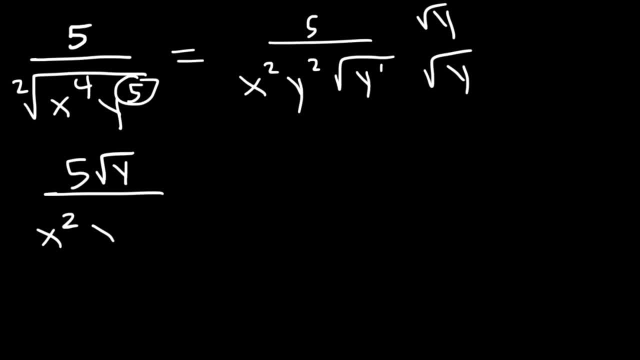 y divided by x squared y cubed. Now the reason why we get y cubed is because the square root of y times the square root of y is y And y squared times y, 2 plus 1 is 3, so you get. 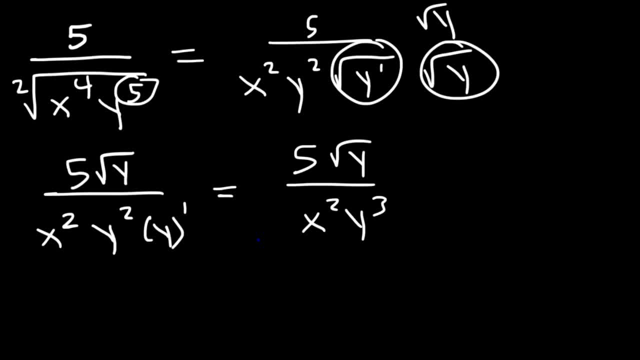 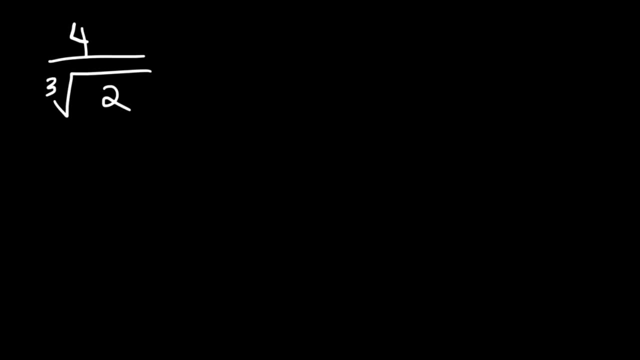 y cubed, And this is the answer. Now let's say, if we have this problem, If we have a cube root instead of a square root, how would you rationalize the denominator? How would you get rid of the radical on the? 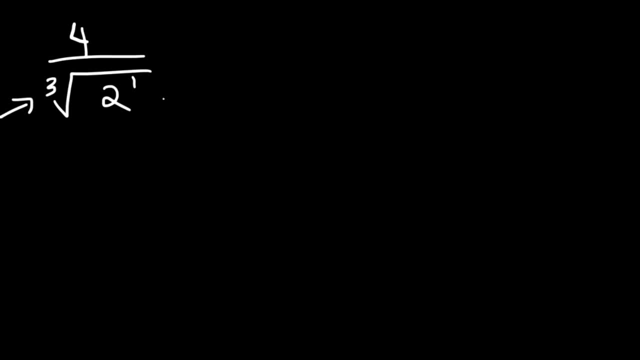 bottom, Because the index number is 3,. to get rid of the radical, we need 3, 2s in the bottom. Right now we only have 1, so we're going to have to multiply the top and the bottom by the cube root of 2 squared. 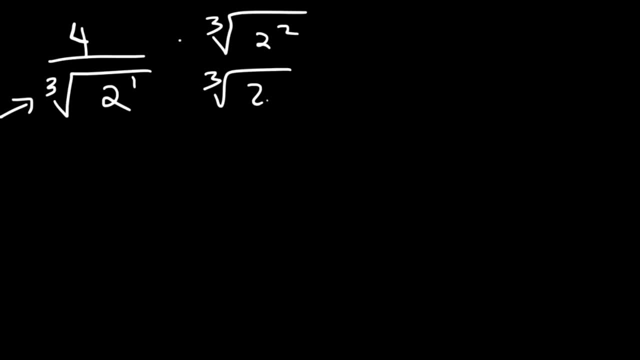 Subtitles by the Amaraorg community. If we do that, on top we're going to have 4 times the cube. root of 2 squared is 4.. And on the bottom, 2 to the 1 times 2 squared. if you add the exponents you're going to get 3.. 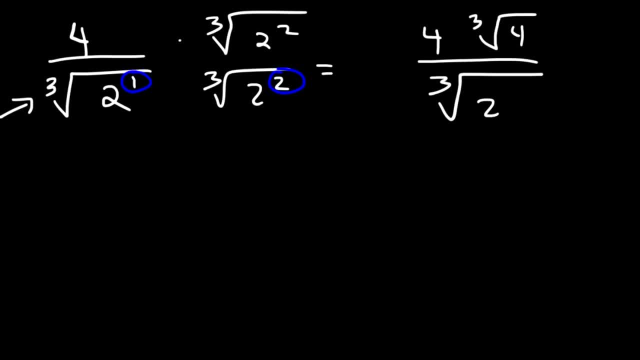 So this is going to be 2 raised to the third power, which is 8.. And the cube root of 8 is 2.. So when you simplify it, these two basically cancel, And so what we now have is 4 times the cube root of 4 divided by 2.. 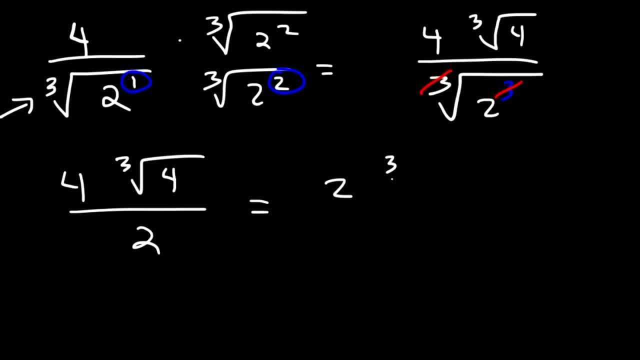 And 4 divided by 2 is 2.. So this is the final answer. Try this one: 3 divided by the cube root of 4.. What would you do in this example? Well, notice that we can simplify the bottom first. 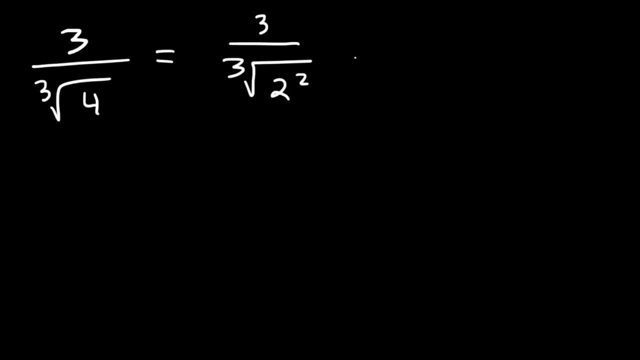 4, we can write it as 2 squared, So we only need one more 2 in the bottom, Because, if you think about it, the cube root of 8 is 2.. So we just need to get to 8.. 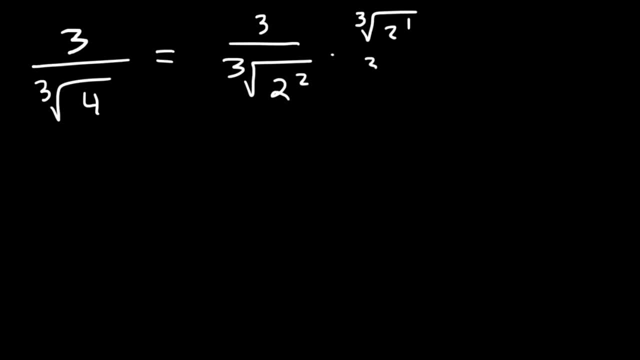 So let's multiply the top and the bottom by the cube root of 2 to the first power. So on top we simply have 3 times the cube root of 2.. On the bottom, we have the cube root of 2 to the third power, which is just going to be 2.. 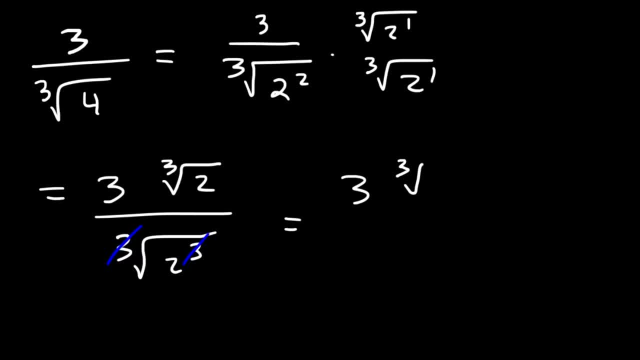 So the final answer is 3 cube root of 2 divided by 2.. And that's it. Try this one Now. for this problem. we have 2x to the first power. So once again we're going to multiply the top and the bottom. 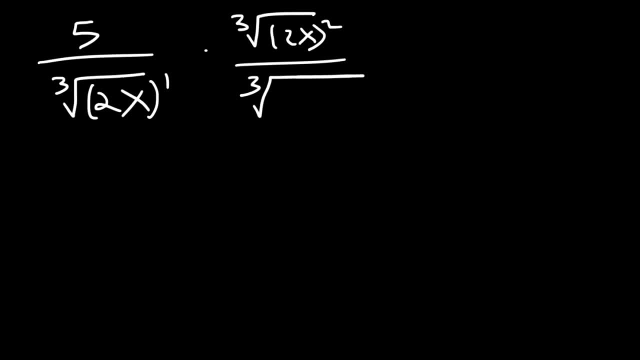 By the cube root of 2x to the second power. So we can have 3 2x variables on the bottom. So on top this is going to be 5 times the cube root of 4x. squared On the bottom the cube root of 2x to the third power is just going to be 2x. 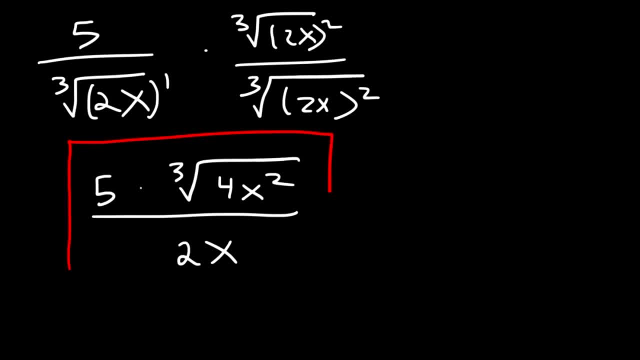 And there's nothing we can do to simplify this fraction. So this is the. This is the answer. Try this one: 9 divided by the fourth root of 3x. In this case, we need to get 4 3x's in the bottom. 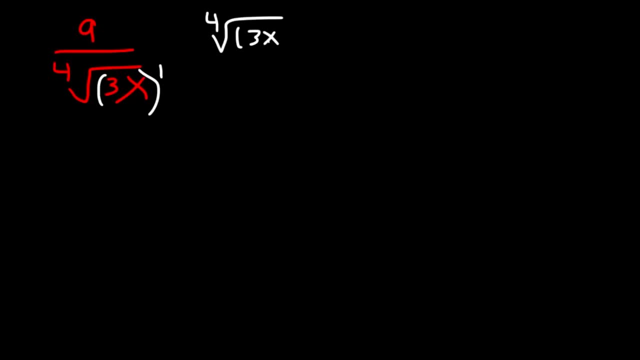 So we've got to multiply by the fourth root of 3x to the third power, So on top that's going to be 9.. Fourth root 3 to the third is 27.. So it's 27x cubed. 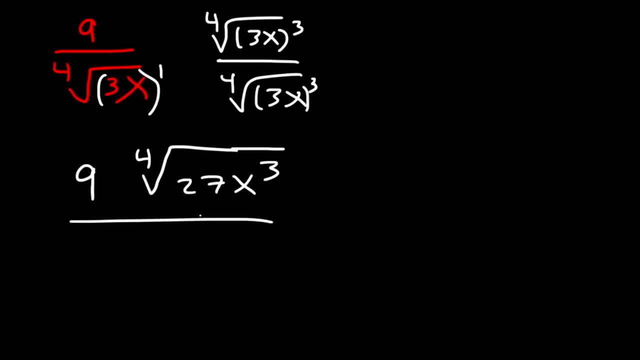 On the bottom. we now have 4 3x terms, So it's just going to be 3x in the bottom, And now we can simplify: 9 divided by 3 is 3.. So then, this is going to be the final answer. 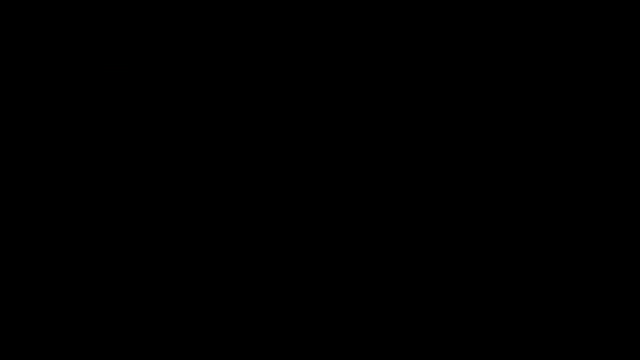 Now let's say, if we have this expression, 8 divided by the fourth root Of 32x. Now, in this case, you want to simplify. first, You can break up 32 into 16 times 2.. Because the fourth root of 16 is 2.. 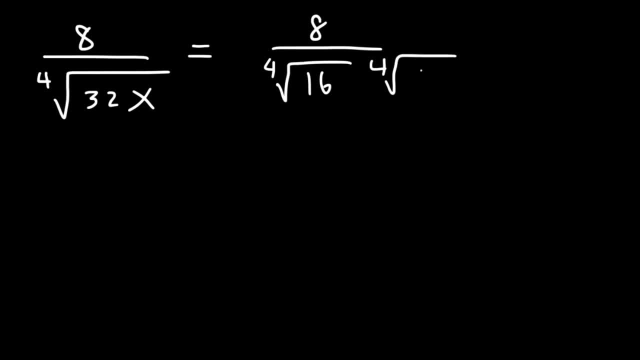 2 times 2 times 2 times 2, four times is 16.. So if you could simplify before rationalizing, do that. So this is going to be 2 times the fourth root of 2x, And 8 divided by 2 is 4.. 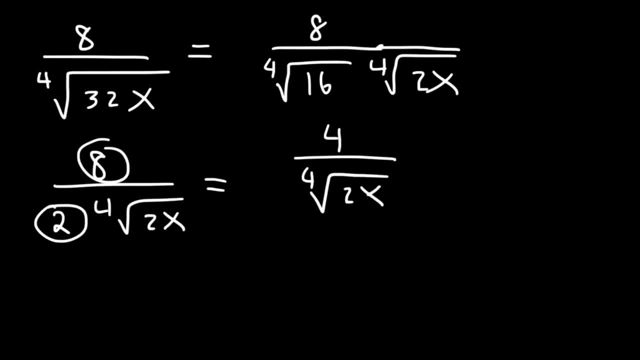 So we have 4 divided by the fourth root of 2x. And now let's rationalize it. So we need 3 more 2x terms. So let's multiply the top and bottom by the fourth root of 2x to the third power. 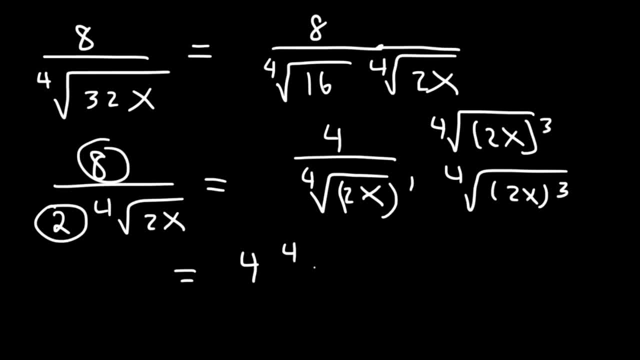 So on top we have 4 times the fourth root of 8x cubed And on the bottom it's just going to be 2x, And 4 divided by 2 is 2.. So the final answer is 2 times the fourth root of 8x cubed over x. 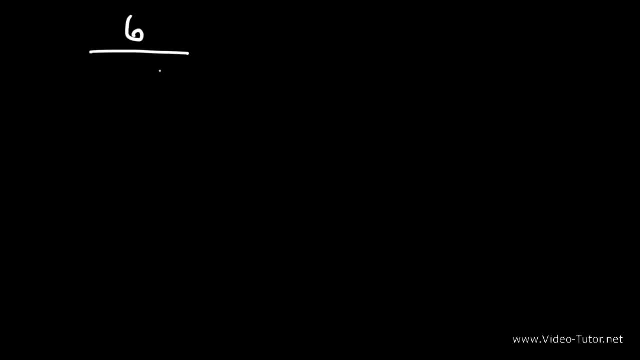 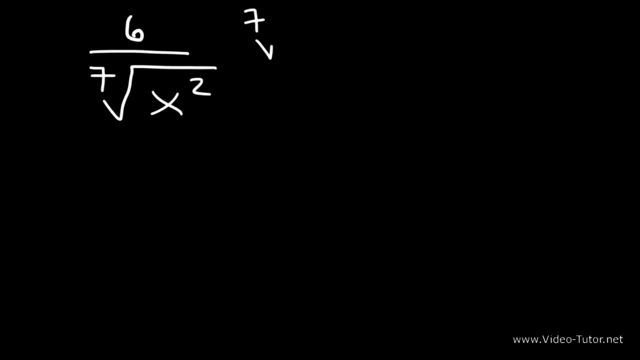 So we need 7.. So we need 7.. So we need 7.. Let's multiply the top and the bottom by the seventh root of x to the fifth power, So on top it's just going to be 6 times the seventh root of x to the fifth power. 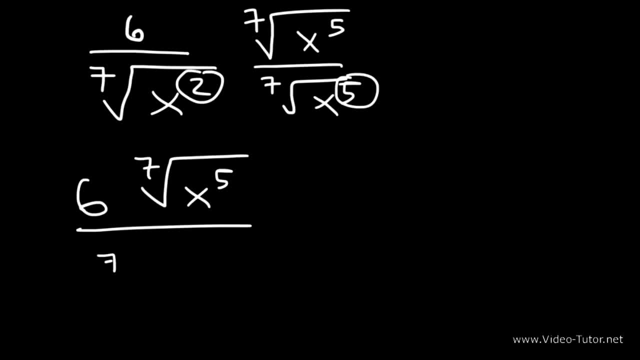 On the bottom, 2 plus 5 is 7.. And 7 divided by 7 is 1.. So the final answer is 6 times the seventh root of x to the fifth power, to the fifth over x, and that's it.